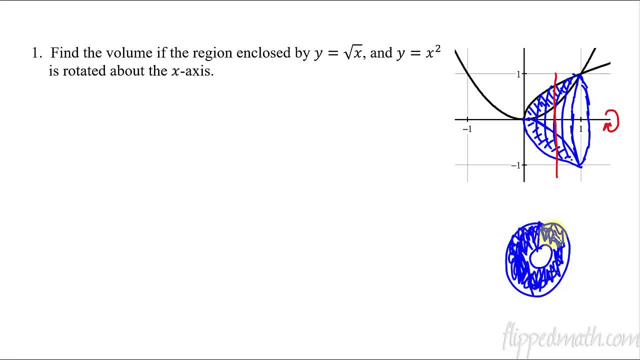 Think about when you put something together, like if you have a bicycle and you're putting the bolts back on a bicycle, you have a washer that goes underneath it. So these washers, or you're putting something together from Ikea, you have this washer goes underneath the bolt or the screw that goes on, and that has a hole in it. That's why this is called a washer method, because when you take a cross section and look at it, it's a washer. Whereas before, our other lessons, what we did is it would just be a full circle, and that was considered a disc method, because it just looks 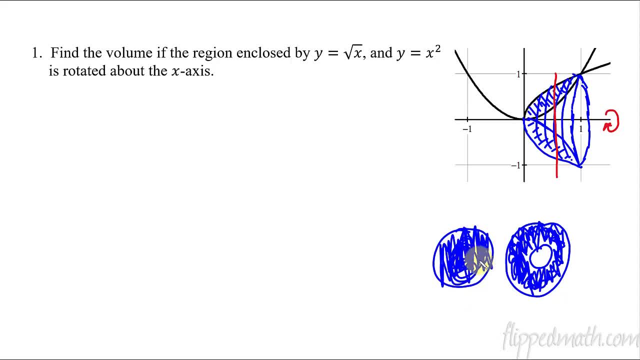 like a solid disc. Okay, so before the last couple lessons, we did discs. Now we're doing washer. 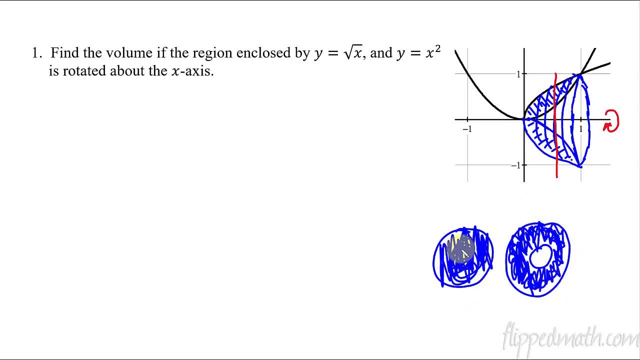 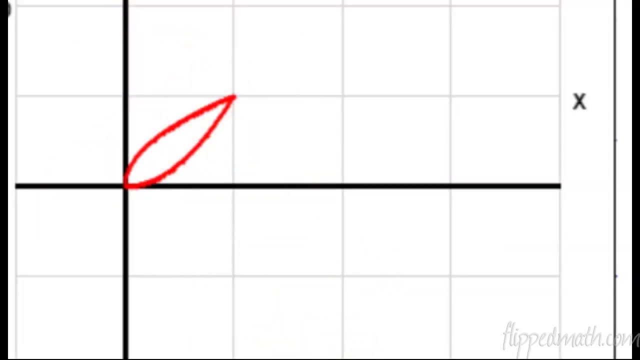 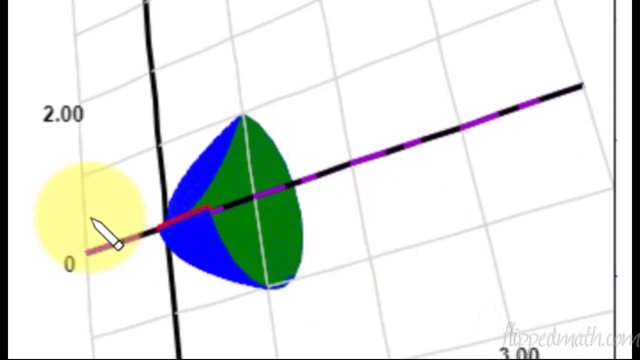 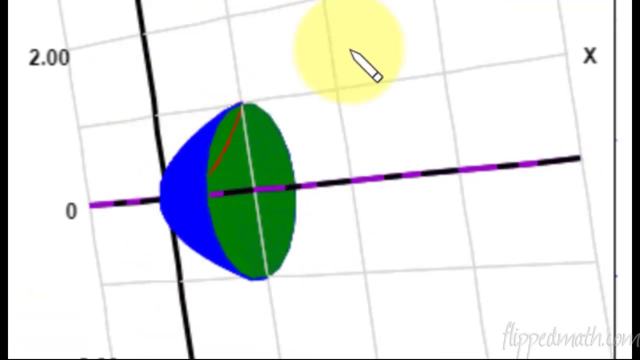 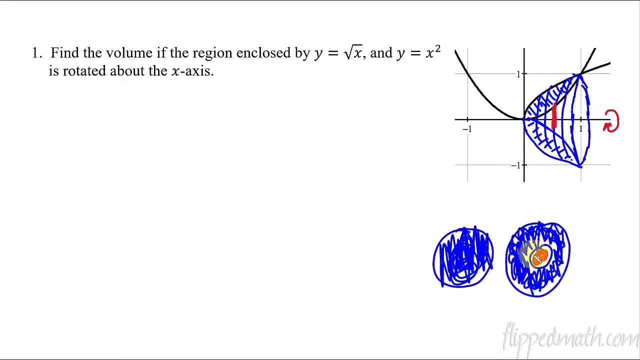 The only difference is you do the whole thing like a disc method, and then you just have to subtract this thing right here, what's in red. I subtract the missing gap. So in here, on my, line here, get rid of this red, that would be this part of it right here. So what's in red is the missing. Let me show you on a little applet what I'm talking about. So here I have the exact same graph, that's the region, and as I revolve this, it revolves, and that's kind of hard to follow, but you can see there's that, just that one piece of area is revolving around. Let me do that again and move it this way just a little bit so you can see. So you can, it's kind of hard to tell with just this, but you can see it's just the outside piece of it. It's not solid. There is a hole inside there. So if I slice it right down the middle of this thing, take a little slice, you'd see there will be a gap on that. So let's set up the volume integral. 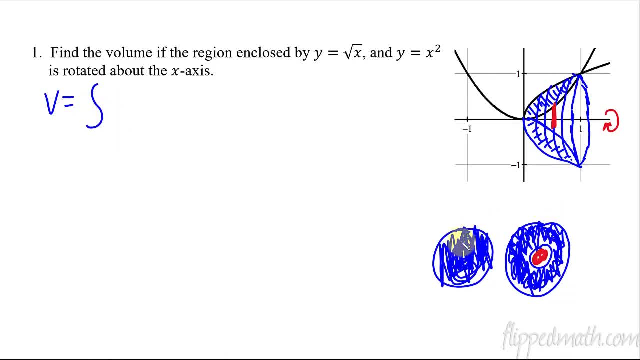 So volume is going to be, let's do the whole thing first. So like we're doing the disc method. So we'd go from what's my re my boundaries are from zero to one for the X value. So zero to one, and then I do pi R squared. So my radius squared is this outside of the object. Which one is that one square root or X squared? That's the square root. So this right here is my capital R, my big radius. So I'm going to say the square root of X squared with respect to X. So I just took the volume of the whole thing. So that would be like the disc. Now I need to subtract what's on the inside, the missing piece in red. So I want to subtract the volume from zero to one of this other little, uh, curve revolved around. In a circle. So pi R squared, but in this case, it's going to be a little R because it's the small radius it's to the inside of the object of what we're missing, where it's just going to be air. It's a gap. So that's X squared with respect to X. Now we can simplify this down more. 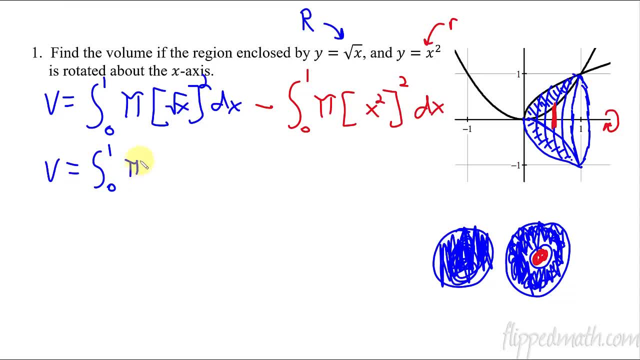 So volume is going to equal zero to one pi of square root of X and squared is just an X DX. 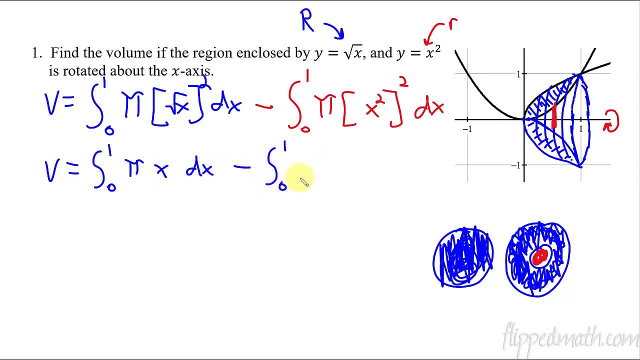 Minus zero to one. And then this is pi X to the fourth DX. Now, when we both, when you have pies on both of them and they're both integrated from zero to one, what we really can do is simplify this to the following. So this is the last part for this. We're not going to actually find the volume. I just want you to set it up on for the lesson in the practice, you will find the volume. So be aware of that. You have to do the anti-differentiation. So here we go. Uh, pi, I can pull to the front. Let's pull the pi in front of the integral. 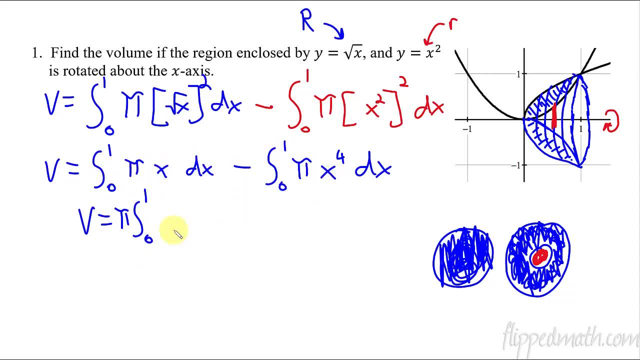 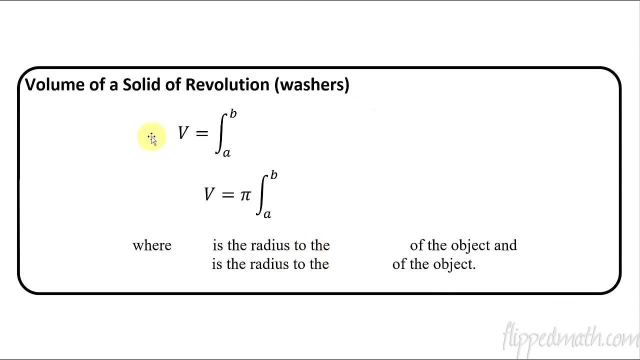 And then I go from zero to one. So it's almost like you're just combining these two integrals. And then what do I have? I have an X minus the X to the fourth with respect to X. So it all becomes one integral. Since I'm integrating from zero to one, they both have pies. I can just put it all together. So that leads us to, uh, the formula for volume of a solid when there is a missing gap right there. That is this. So we just did this part. We take pi big R squared, minus, and then the same integral from A to B of pi little R squared, little radius. And then you can combine that to this thing. You have the capital R squared minus little R squared. And here's what our big R and little R stand for. The big R is the big radius. It goes to the outside of the object that we're revolving. And the little R is the small radius. It goes to the inside of the object, most textbooks, and most teachers will just teach this, which is absolutely fine. I like to focus on this one. So I'm going to go back to the first one. I'm going to go back to the second one. 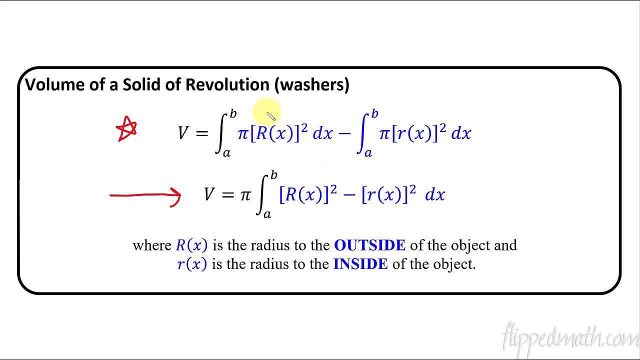 First, because it helps you understand that you're doing the radius of each one separately. You're finding the volume of the whole thing, and then you're subtracting the volume of the little thing, the little radius. The reason I say that is because the most common mistake I see on these is not squaring the radius individually. Let me repeat that because you might want to rate, write that down. The mistake is making sure, or excuse me, not the mistake, but the thing that you need to do is square each radius individually. Do not do a quantity squared. This is the mistake where they do this little R of X of X, big R of X minus little R of X quantity squared. That is wrong. Don't do that. Okay. This is what it's supposed to be. Little, a big R squared minus little R squared with respect to X. Notice where I put the pie. Don't lose track of that pie, that pie. I just put on the outside, uh, because, uh, you know, you're allowed to take the constant to the front, which is fine. Just don't forget about it. When you're done, multiply by the pie. 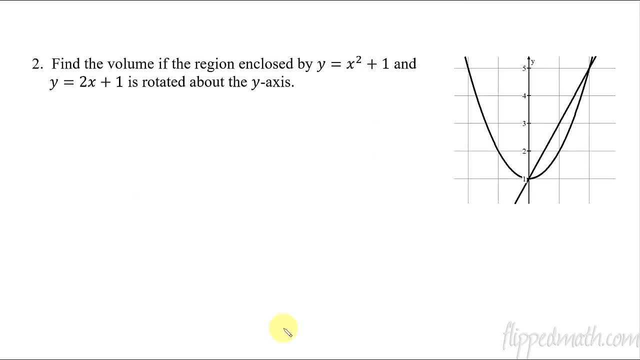 That's another common mistake. Okay. Our lesson's pretty much over. Let's just do one more example real quick with respect to why. And then I think we're good. So here we have this region. Let's figure out what the graph is doing. We are going to have to draw this line here, do the mirror image, and we're going to revolve this this way. So I'm going to make a kind of a oval shape. Oh my goodness. This is hard to use this electronic pad, messing this up. Okay. So there's our shape and you can see the open white space here. This is the hole. If we do the cross section, you'd have the washer. This is the open gap. Now, since we're doing it on the Y axis, we need equations with respect to Y. So Y minus one equals X squared. Take the square root of both sides. It is going to be a plus or minus Y minus one equals X, but I only want this right side, right? I'm just doing this one. That's the one that I started with and I'm revolving it. So I can just say that X is equal to the square root of Y minus one. 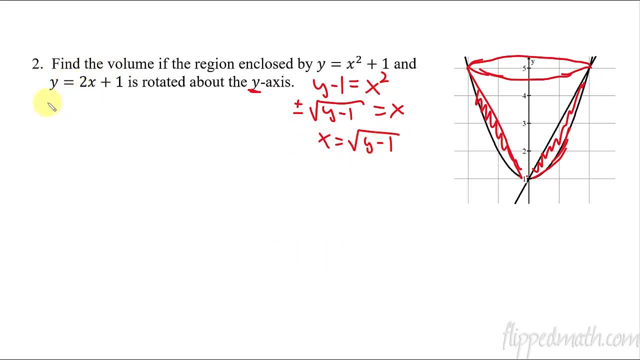 And then how about this one? So let's solve for get X by itself on this one, Y minus one, and then divide everything by two. I get Y over two minus one half equals X. All right, let's set her up. So I take pi and then I go from the lowest Y value. The lowest Y value is right there. That's a one to the highest Y value. The highest Y value here is a five. And then I need 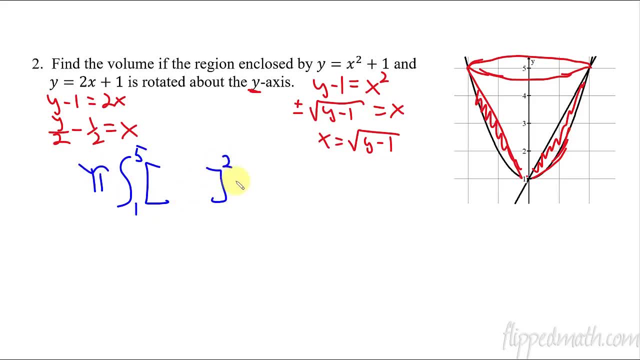 to do this because I already put it out front. So my big radius squared minus my little radius squared with respect to X. So what is the big radius? The big radius, I'm going to go from the middle of where I'm revolving to the outside of the object. That's the big radius. What's the curve on the outside of the object? That is the curved one. So which one's that one? This one. That is my big R. So that's the square root of Y minus one. 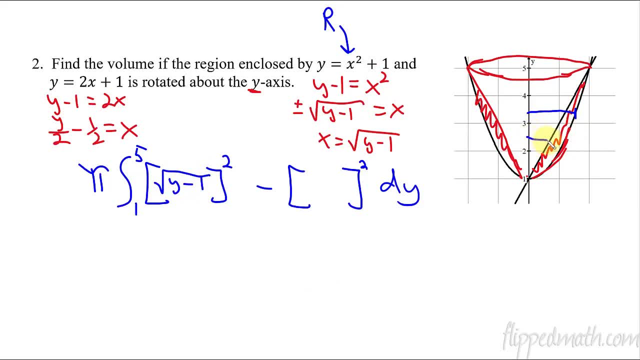 And then my little R is to the inside. So that's my big R. That's my little R. My little R is just there to the inside of the object, which in this case is this one. There's my little R. And so that 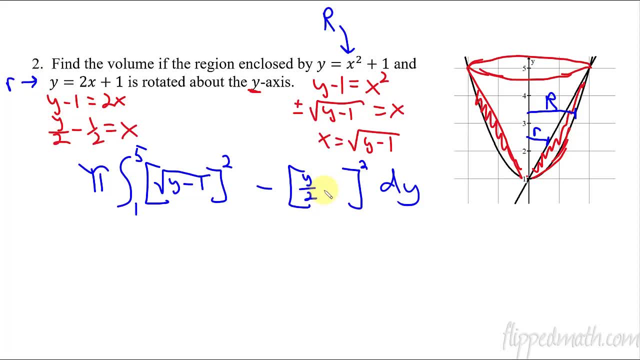 solved for this. So I have Y over two minus one over two. And then there's my answer. This is it.